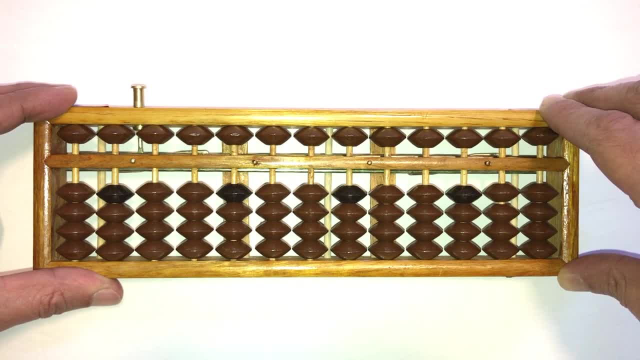 and sharpen this ability to visualize and easily calculate large string of numbers. Now, this amazing and powerful capability not only helps them in math, but also improves their focus, their concentration, memory, their attention, which, incidentally, helps them not only in school. 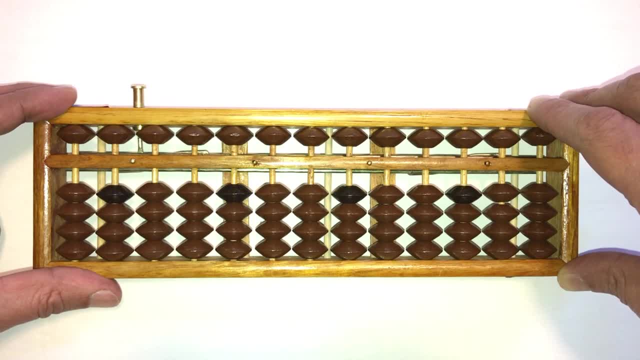 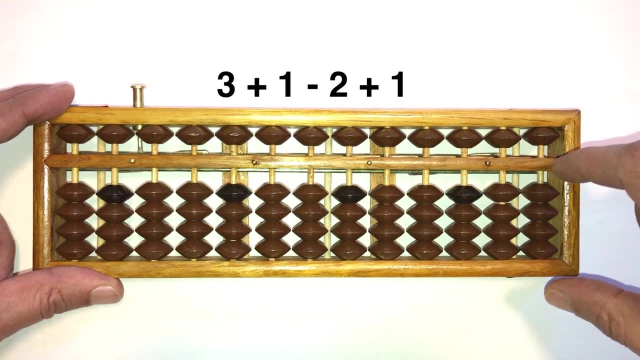 but also with other creative pursuits like music and art. Well, with that in mind, let's dive in. Let's solve: three plus one minus two plus one. Three plus one. What do you see touching the answer bar? I see a four. Take away two, Add one. 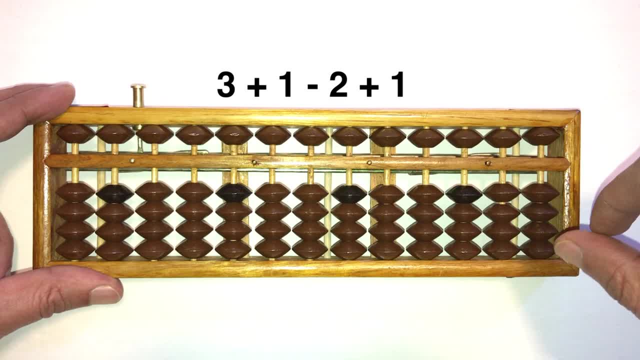 What's left touching the answer bar now, It's a three. Let's do that again. Let's do three plus one. Take away two, Add one. The answer is three. Well, let's do another one. Let's do one plus two minus two plus three. So let's move one up. 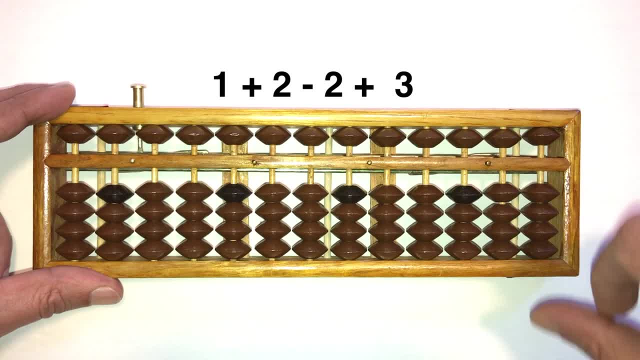 with our thumb. Imagine we just moved one bead up Plus two. I see three now touching the answer bar. Take away two, You're left with a one Add three. Answer is four. Okay, let's do that again: One plus two minus two plus three. Answer is four. 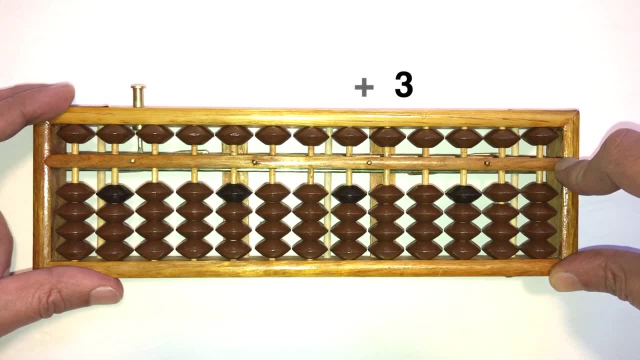 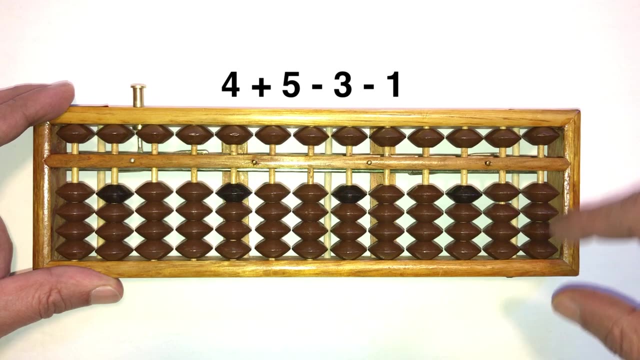 Well, so far we did lower beads only. Now let's bring in the upper beads. Let's do four plus five minus three minus one. Four plus five. I see a nine now touching the answer bar. Take away a three. Take away a one. 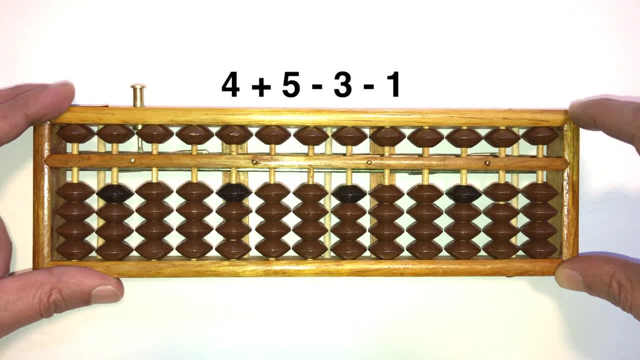 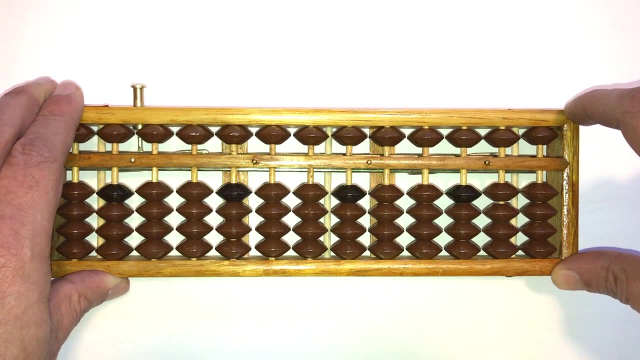 Answer is 5.. Okay, let's do that again: 4 plus 5 minus 3 minus 1.. Answer is 5.. Now let's put the abacus away for a minute and just visualize the abacus in our mind while moving our fingers to pretend. 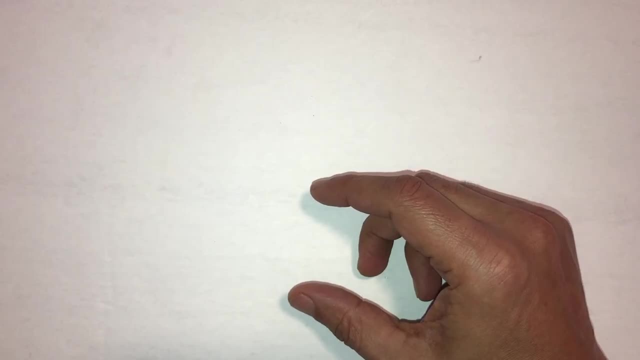 that we're moving the beads. Let's solve 1 plus 2 plus 1 minus 3.. So now we don't have an abacus there in front of us, We're just going to imagine that we're moving beads in the ones column and 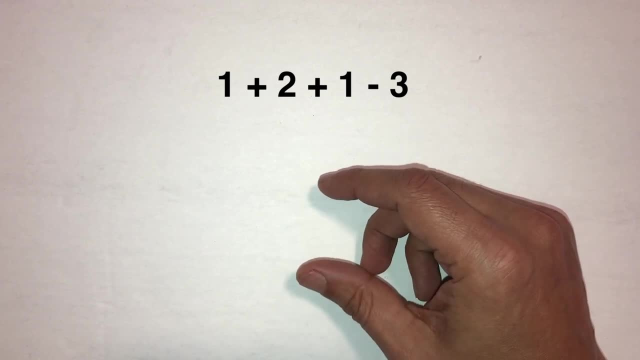 coming up with the answer. So here we go: 1 plus 2 plus 1. Take away the 3. Answer is 1, right, So let's try that again: 1 plus 2. We see a 3 touching the answer bar in our mind, Plus 1.. Now 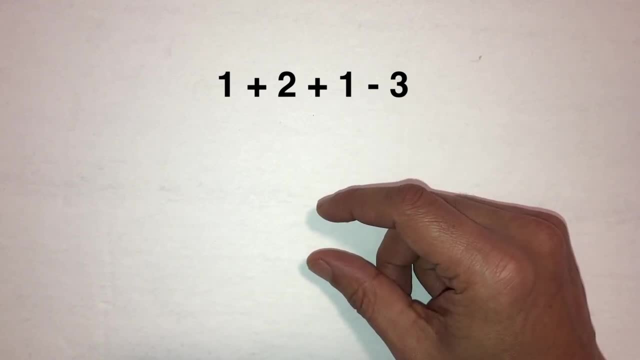 we've got a 4. We take away the 3. We're left with a 1. That's why the answer is 1. Let's do another one. Let's do 3 plus 1 minus 2 plus 1. So here we go: 3 plus 1. We see a 4. 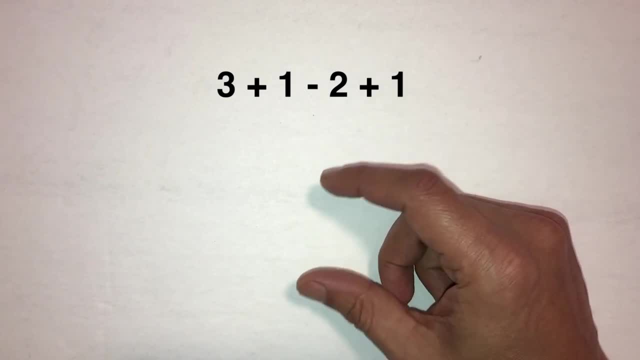 touching the answer bar. Take away the 2.. We've got a 2 left. Add a 1. 3. Okay, Here we do that again: 3 plus 1 minus 2 plus 1.. Answer is 3.. Now let's bring in the upper beads, Let's do 5. 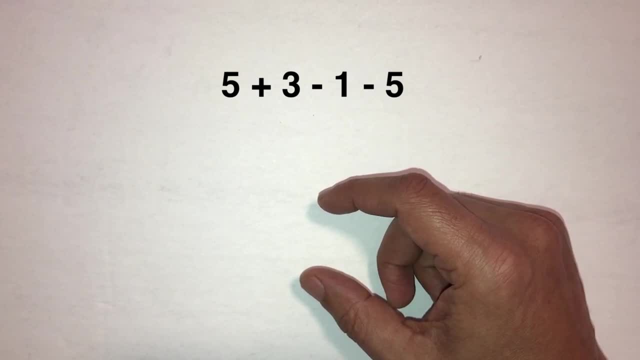 plus 3 minus 1 minus 5.. So 5 plus 3.. We've got 8.. Take away the 1.. Take away the 5.. We've got a 2 touching the answer bar. Let's do that again: 5 plus 3.. Take away 1.. Take away 5.. 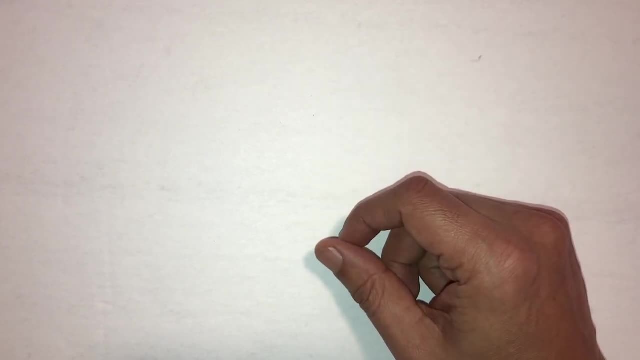 The answer is 2.. Now let's try another one with the upper beads: 3 plus 1 plus 5 minus the 4. We're left with the 4. 5.. Do that one again: 3 plus 1 plus 5 minus the 4. Answer is 5.. 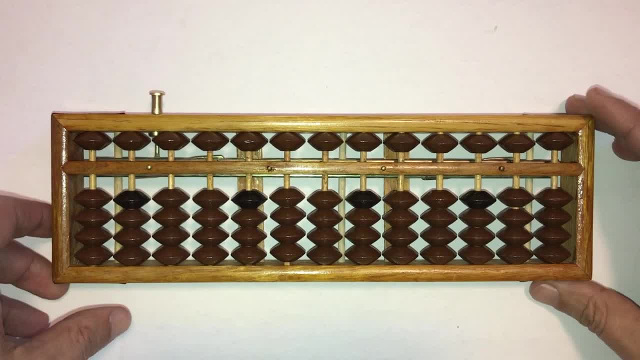 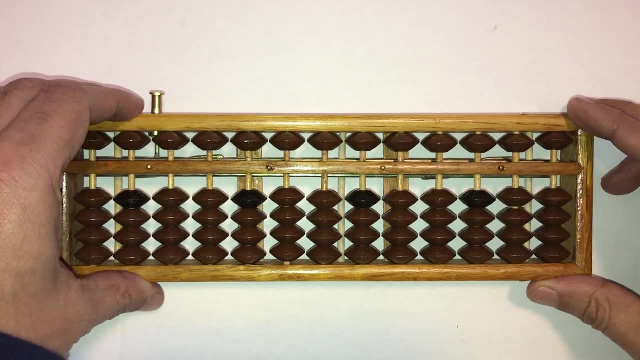 Now there are several reasons why, during mind math, we ask students to move their fingers to mimic what they would do if they were moving the beads on a physical abacus. Two key reasons among them are that, first, it maintains their focus and helps them better visualize, and secondly, as 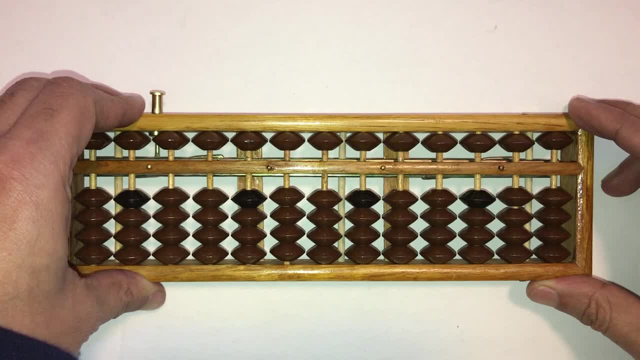 teachers. it demonstrates to us that a student is actually visualizing the beads and not taking shortcuts by solving using traditional math. If we don't develop this ability to visualize early in the program, students generally struggle as questions get harder. Now, in any case, as the 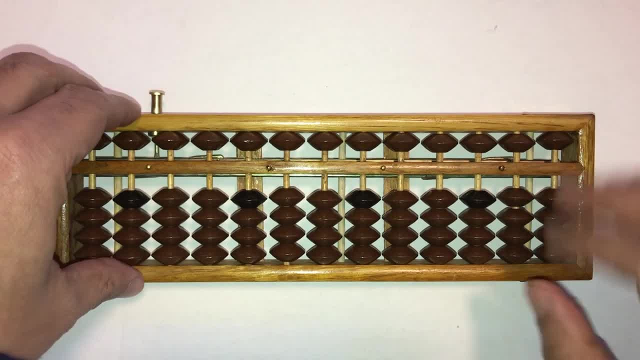 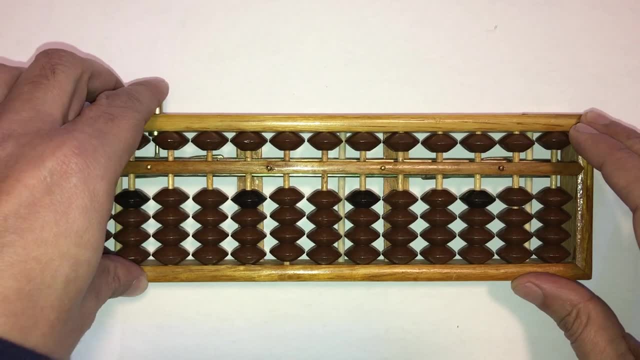 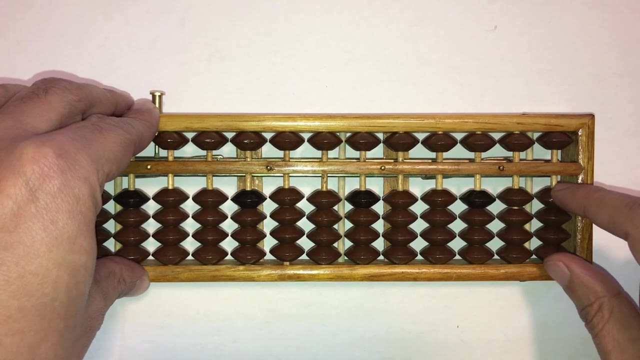 student continues to improve, visualizing just becomes second nature and they can stop using that finger movement during mind math. Let's talk about worksheets really quick. If you, If your student is 5 or 6 years old, focus only on the MindMath worksheets with lower beads in this lesson.